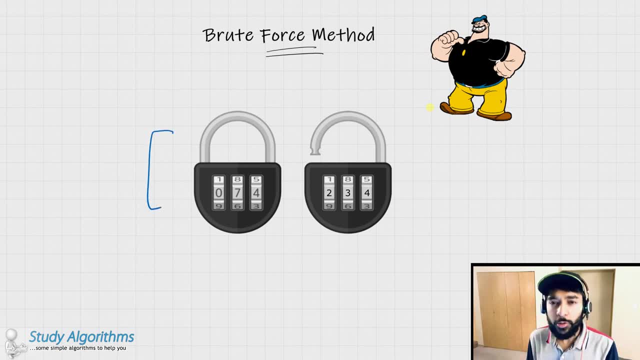 a padlock. You must have seen these kinds of padlocks in day to day life. So this one can be opened using a three digit combination. Now this has a combination of two, three, four. If you know this combination, then it is fairly simple to open it. 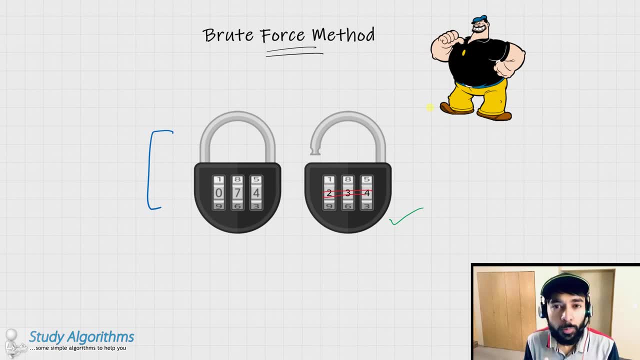 But what if you don't know this combination and you still want to open this padlock desperately? and you're trying that maybe I can just open this padlock somehow. Well, what do you do? One thing that would come to your mind is: what if I try all the? 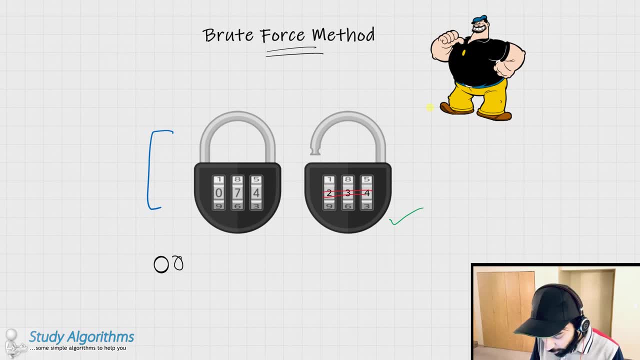 combinations that are possible. So I would go with zero, zero, zero, then zero zero one, zero, zero two, zero, zero, three, and then so on. You get the idea. And eventually what would happen is you would land upon the code two, three, four and this padlock would open. 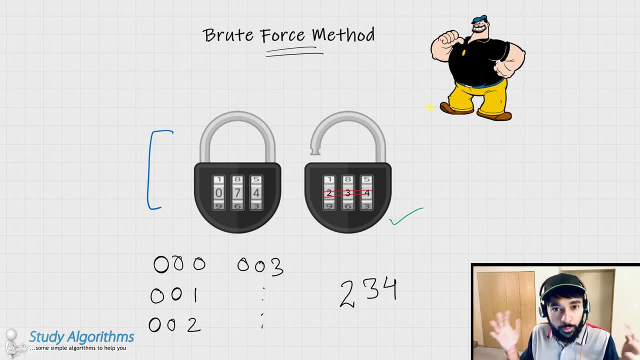 So what did you just do? You just exhausted all of your possibilities to open the padlock, And this exactly is a brute force method. You are deploying all their forces available to you, no matter how much the time, and you're trying to solve a problem. In this case, the maximum number of combinations that 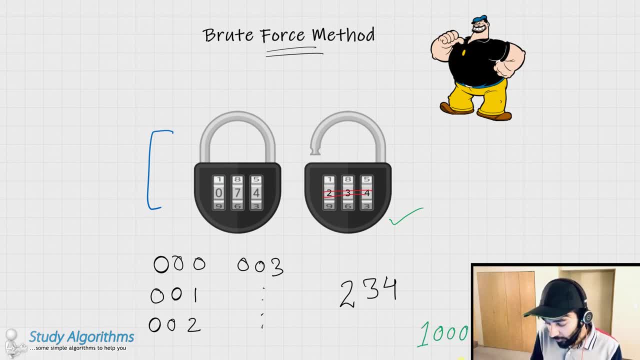 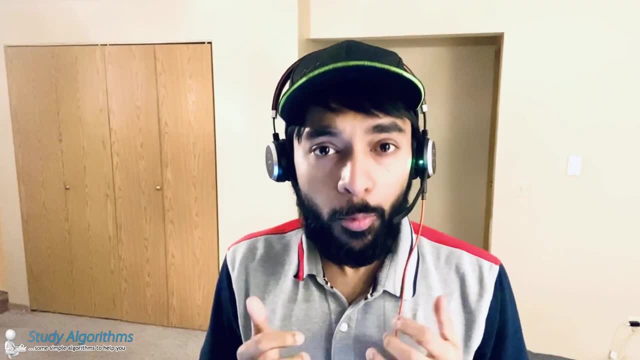 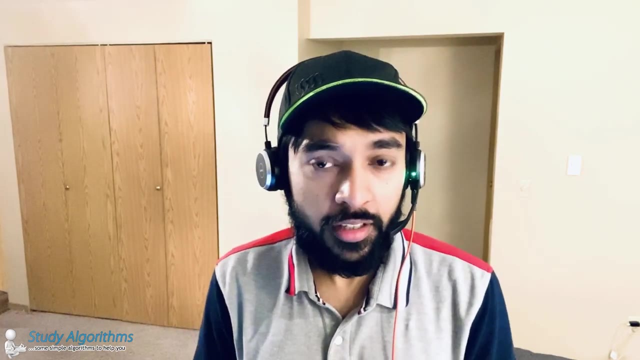 you could have was 1000.. And going on and on and on. you would eventually try to figure it out, But do you see the problem with this method Momentarily? it may see that, given some time, I should be able to solve any problem using a brute force method. 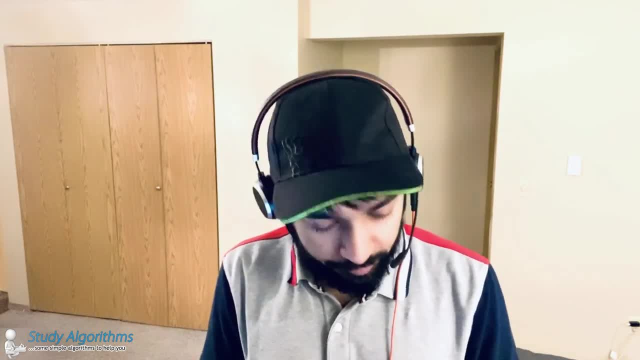 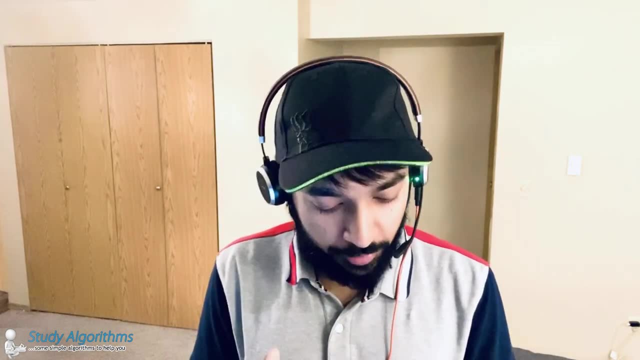 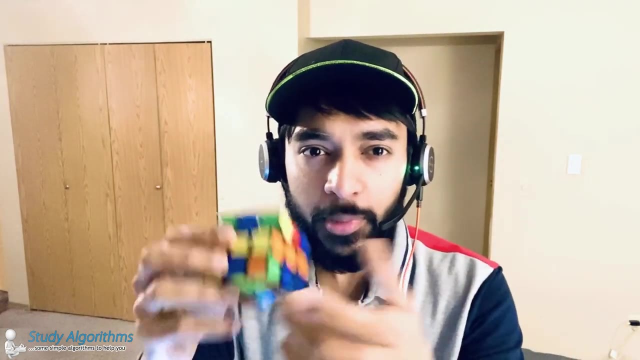 Well, that is true, but it is quite limited. In an earlier example of a padlock, the maximum combinations that we had were just 1000.. Let me take up another problem, And that is some one of my favorite problems of a Rubik's cube. All of you must be familiar with the Rubik's cube. 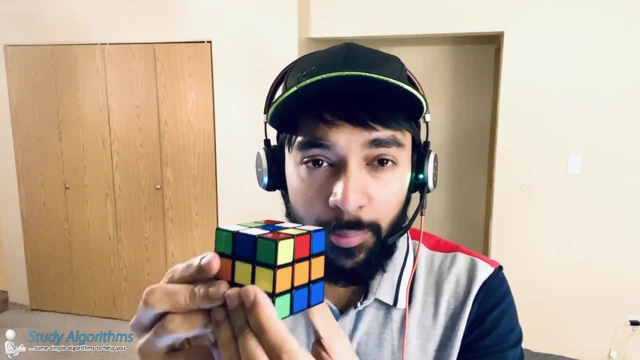 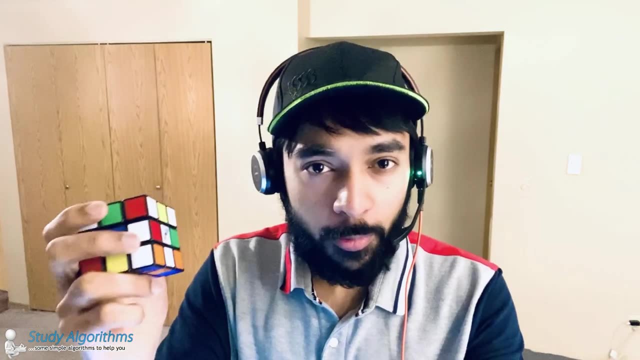 It has got six faces and six colors And ultimately what I need to do is each face should have a single color. You cannot even start to think how many total number of combinations are possible. This, for instance, is one combination If I rotate it in this way. 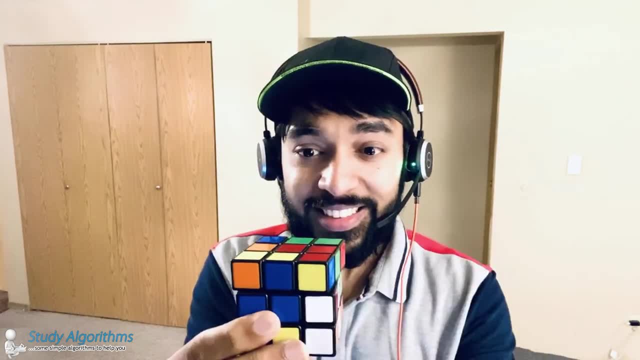 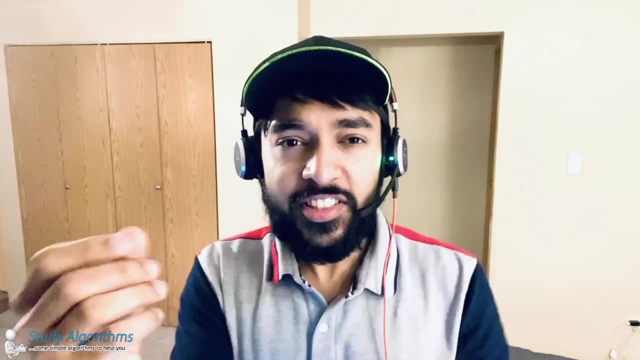 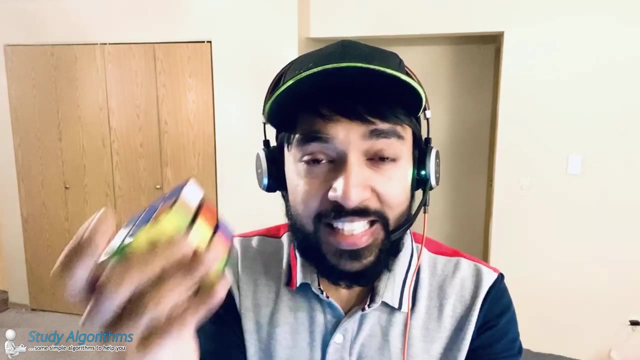 this is another combination. I rotate it another. this is again another combination. In fact, any combination you try, there is a very slight chance that you would be repeating one of your choices, And this Rubik's cube has a total of 43 quintillion total combinations. 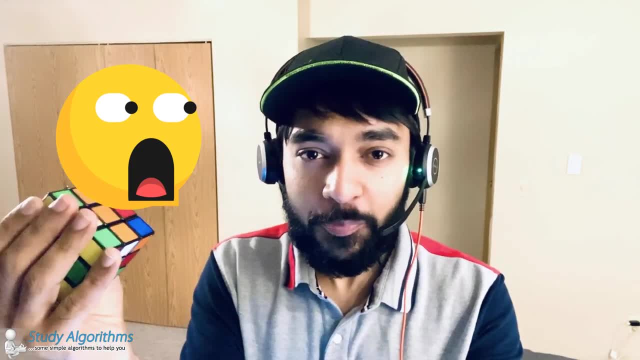 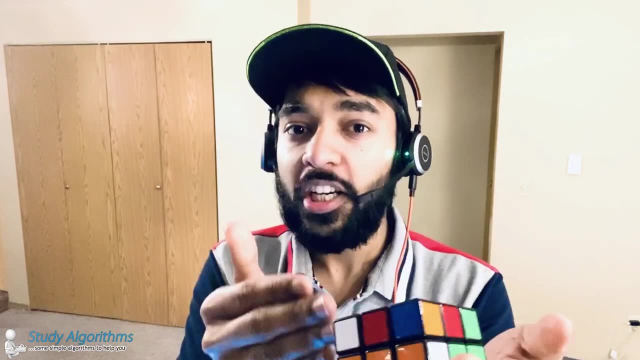 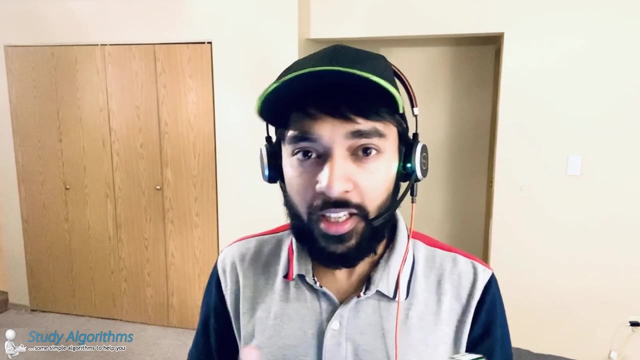 That's like 43 followed by 18 zeros. That's too much, right? So you cannot even hope to solve this Rubik's cube using a brute force method. Yes, given a lot of time, you would eventually arrive at a solution and you would be able to solve it, But that won't be optimal. 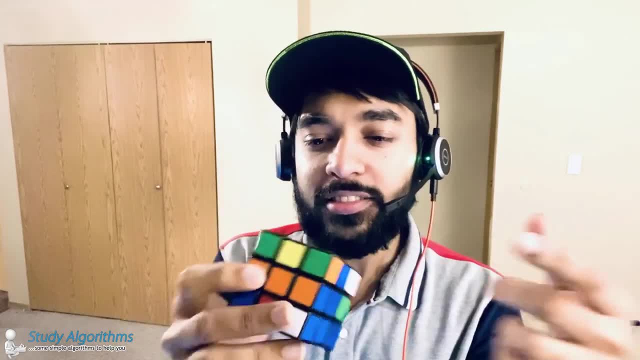 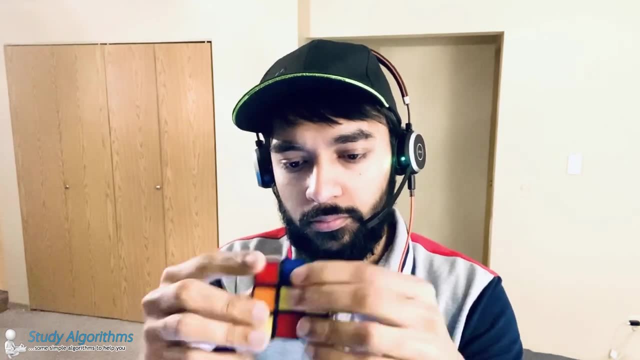 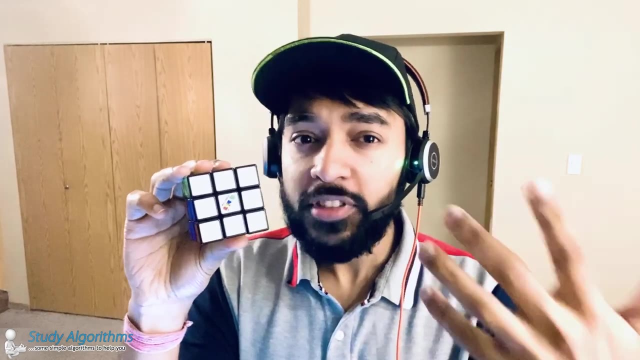 Since I'm a kind of a control freak, I would just go ahead and solve one of the faces for you. As you can see, I actually managed it without involvement, So I made one of the faces. What I did here was I applied some tricks to solve this one face. 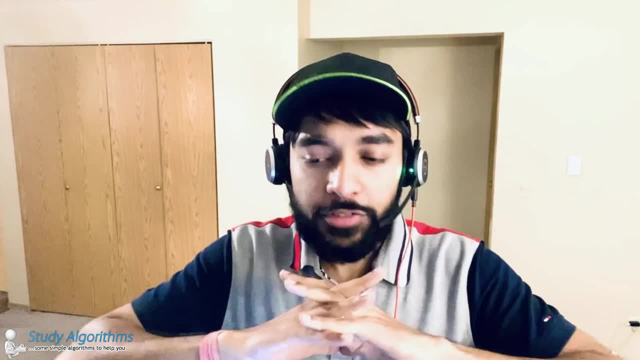 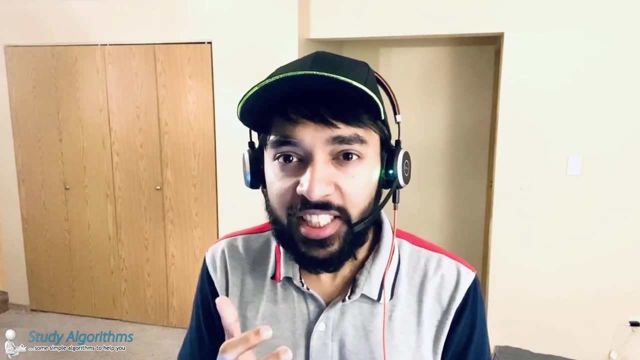 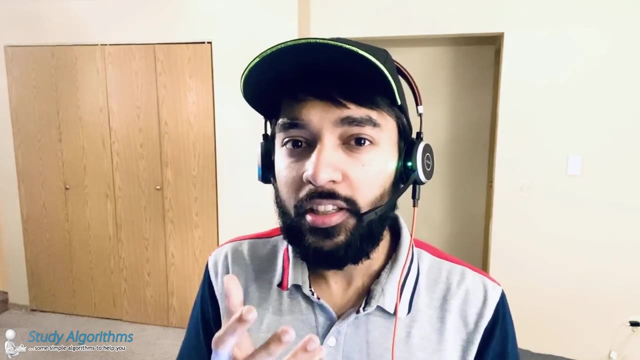 and that is not a brute force method. To summarize a brute force method, what you can say is you're exhausting all of your options to find at a solution. In most of my videos, you must have seen that I always emphasize solution. Why is that so? Let us try to have a look at it. I always emphasize on the fact. 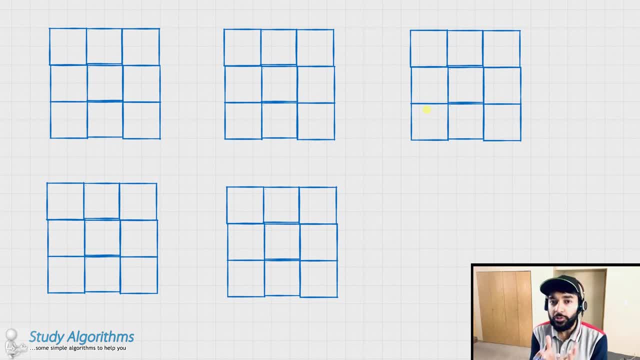 that a good developer would always try to come up with a brute force solution first and then try to optimize it. But why do I say that? That is because a brute force method would guarantee you to find a solution, if that exists. What do I mean by that? Let us take up. 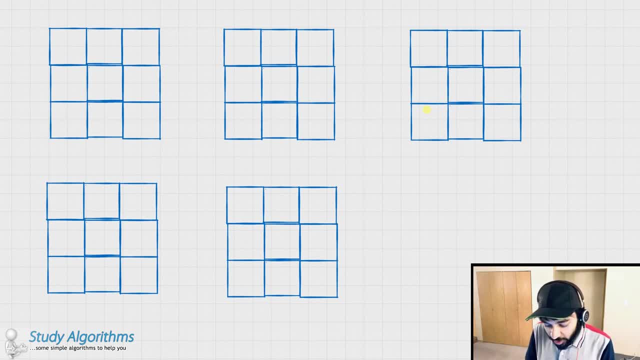 the problem of a magic square. So a magic square is a three by three grid in which you have to fill the digits from one to nine in such a way that some of all the rows, columns and the diagonals are the same. Now how do you go about filling this? A brute force approach would be. you start. 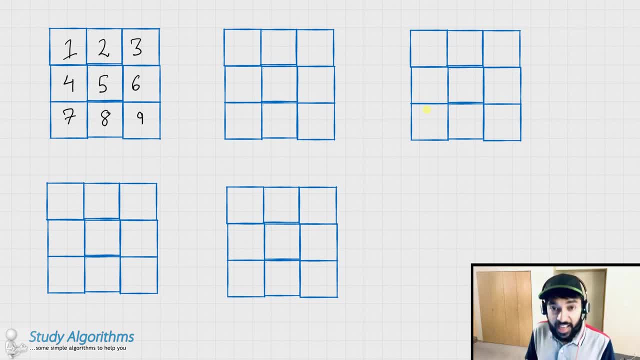 filling of the numbers randomly and then try to calculate the sums of all the rows and columns. In this case, we found the sums to be pretty different, And hence this is not the solution If you just keep on applying the brute force method, something like this: 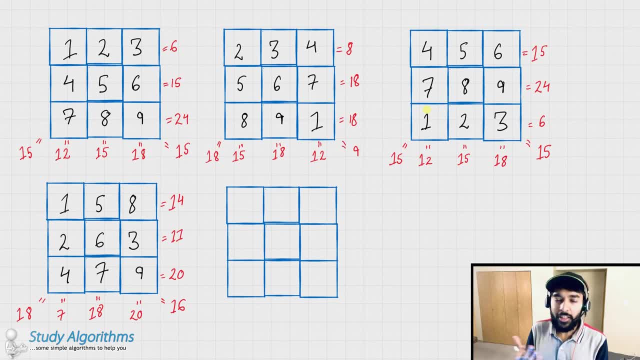 I just took up some random combinations to just find out the sums And while applying all of these combinations, you would eventually- maybe after 32,000 possibilities, you would land up on the exact solution, Which would be something like: In this case, the sum of all rows, columns and diagonals comes out.